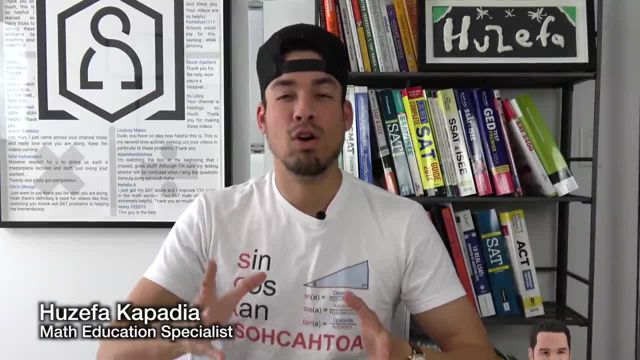 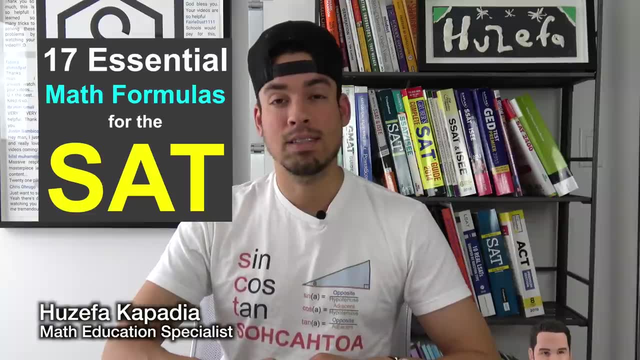 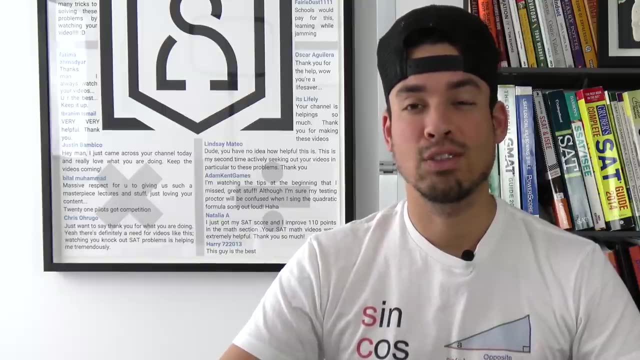 What's up SAT test takers? This video is all about the 17 most essential math formulas that you've got to know in order to do your best on the math section of the SAT. The first formula that you've got to know is how to calculate slope of a line, So that's why we got 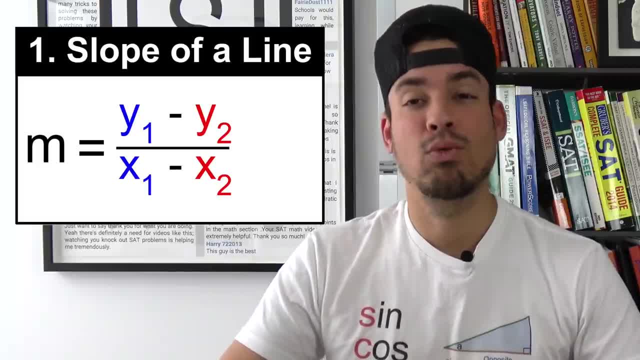 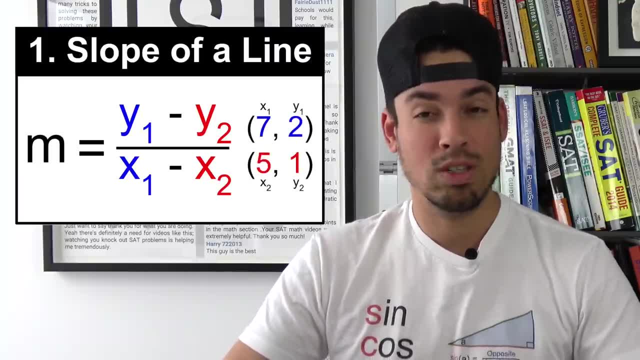 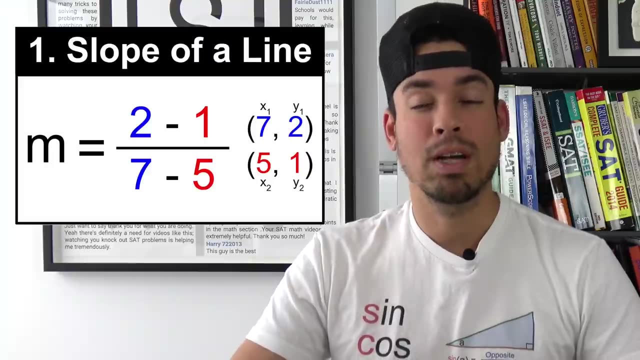 this nice y1 minus y2 over x1 minus x2.. Those are placeholders for values of two coordinates. So all you got to do is pick those coordinates. Doesn't matter which one is y1 or which one is y2.. You just have to choose and stay consistent. The x1 and y1 are a pair and x2 and y2 are a pair. 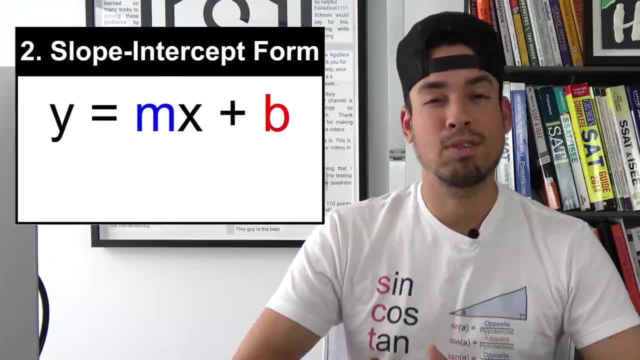 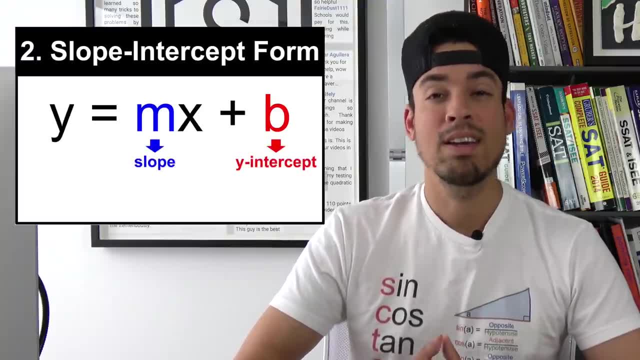 The next formula on this list is slope intercept form. Absolutely critical that you know this formula. The m in the formula represents the slope of a line and the b represents the y intercept. And something super important, when you're given a linear function or linear equation on this test. 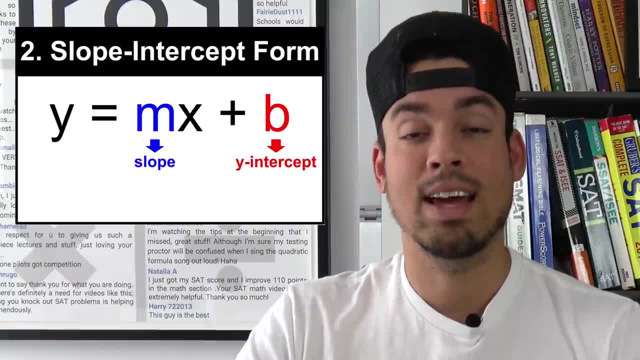 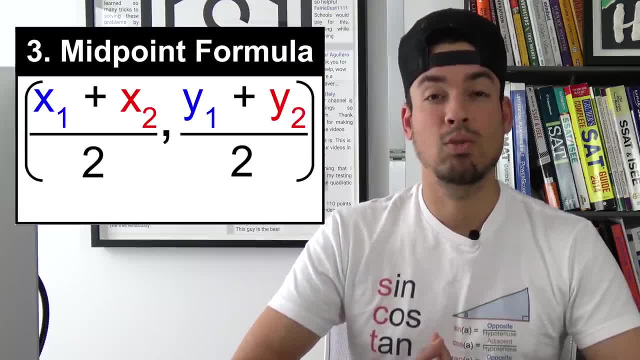 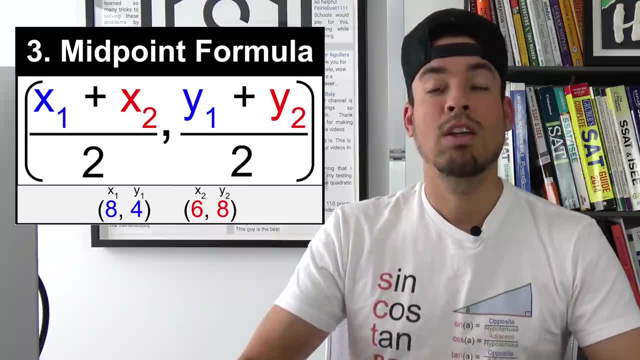 the midpoint formula. This will allow you to find the midpoint between two different coordinates, And if you don't remember it, you just have to know that midpoint is exactly in between two points. So all you're doing is you're taking the average of the two x values and the average of the 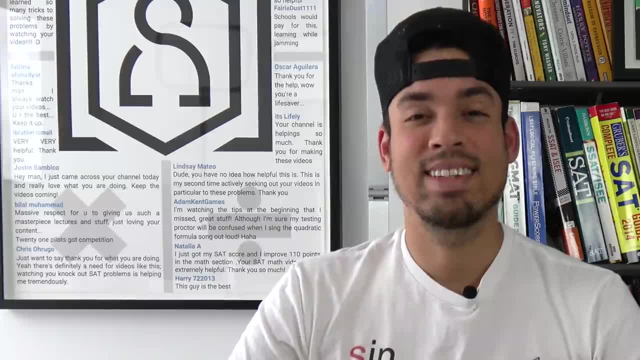 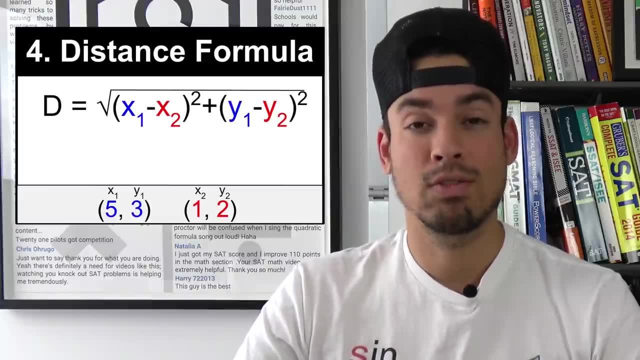 two y values, and that's it. Next on the list is the distance formula. Now, remember, the distance formula is really just Pythagorean's theorem, And if you forget the ins and outs of this formula, you can plot the two coordinates and create a little triangle and 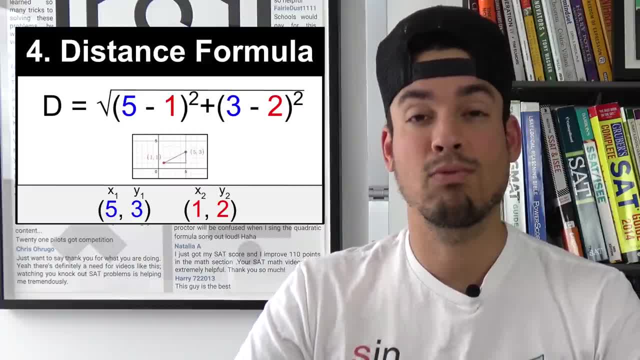 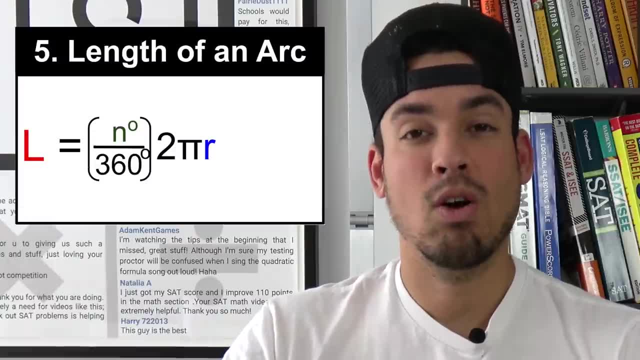 then just calculate the hypotenuse that way. But this is a really important formula and is almost always tested on the SAT. Next on the list is the length of an arc. Now we calculate arc length of a circle, which is kind of like- I consider it- the crust of a pizza. So it's that outside chunk of 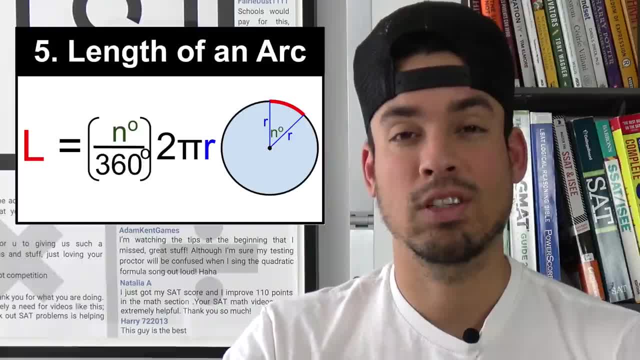 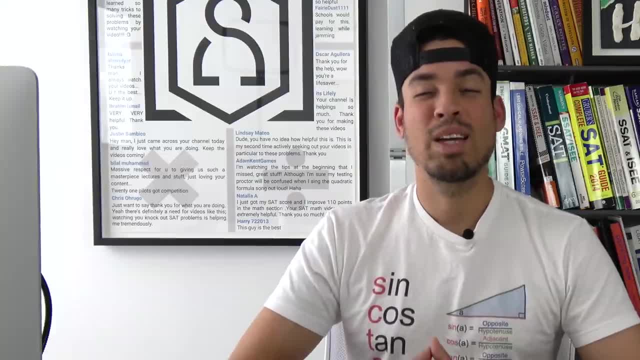 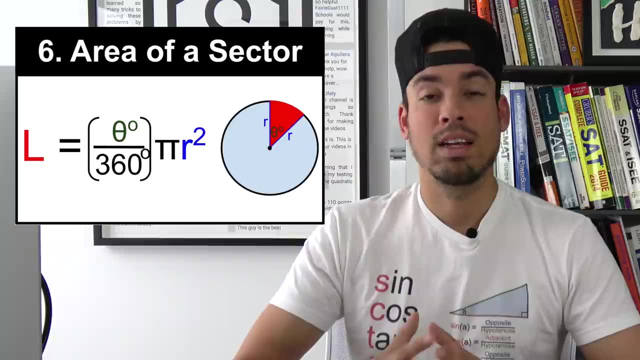 a circle and it's just a length calculation. The n value represents the measure of the central angle and of course r represents the radius. Next we have area of a sector. So arc length is like the crust, area of the sector is like the whole slice of the pizza And the theta in this formula represents the angle, the central angle. 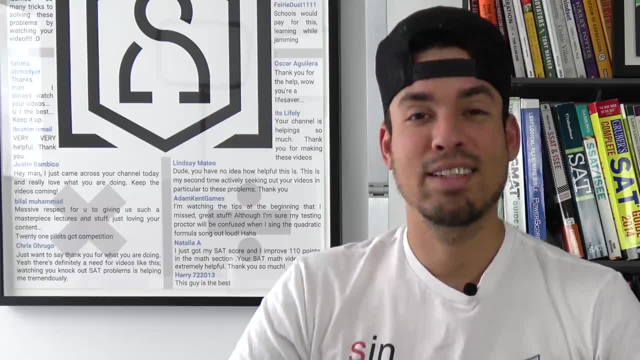 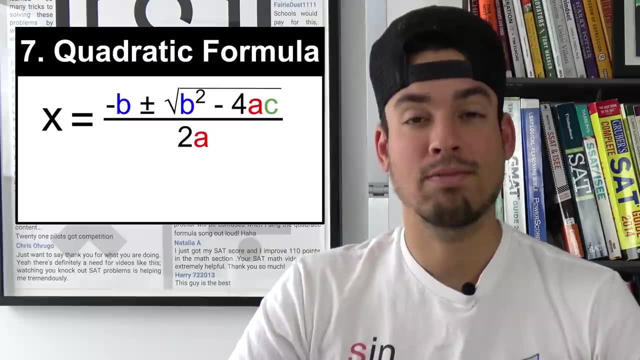 and, of course, r represent radius. Next on the list is the quadratic formula, And now this is a really famous formula and it helps you to find the roots of a quadratic function, which means you're finding the spots where it intersects the x axis. Next on the list is 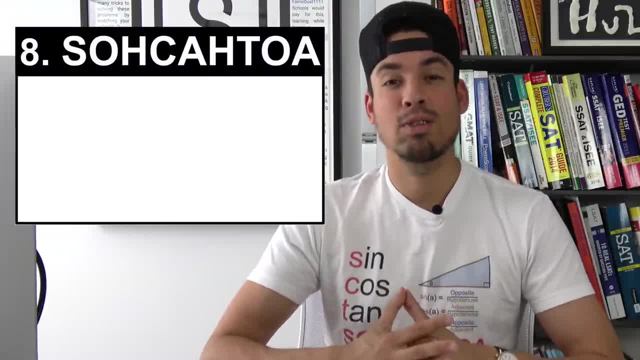 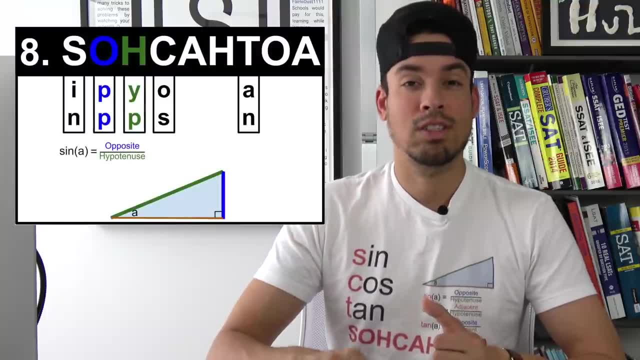 SOHCAHTOA, which of course I'm wearing on my shirt, and that's an incredible acronym to help you remember the ins and outs of the trigonometric functions: sine, cosine and tangent. SOH stands for sine is opposite over hypotenuse, CAH stands. 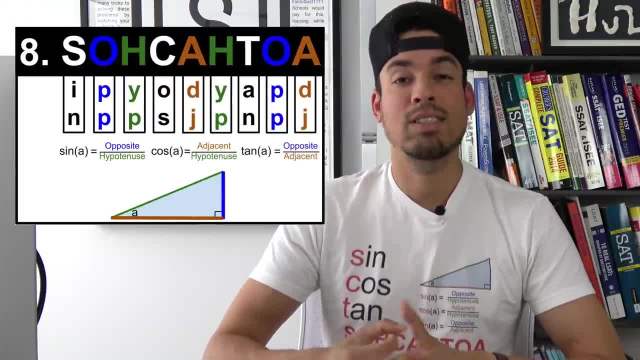 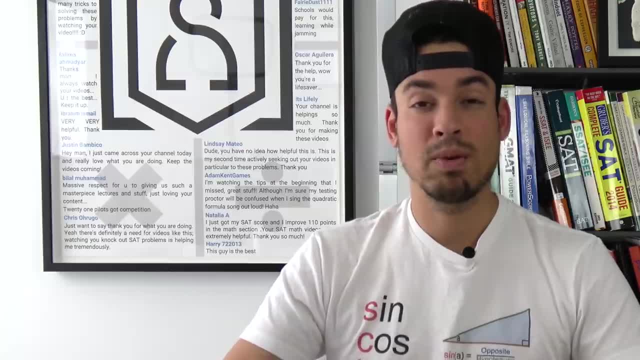 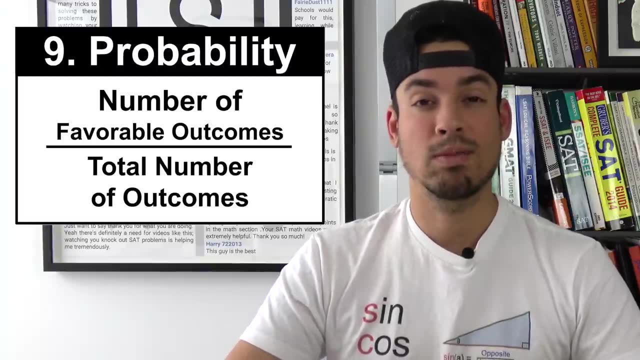 for cosine is adjacent over hypotenuse and TOA stands for tangent is opposite over adjacent. Next on the list is the simple but very important formula of probability, which is the number of favorable outcomes, or aka the number of ways to win over the total number of outcomes. Next we have the equation of a. 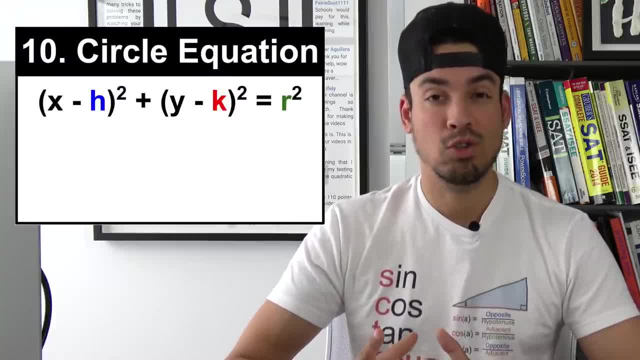 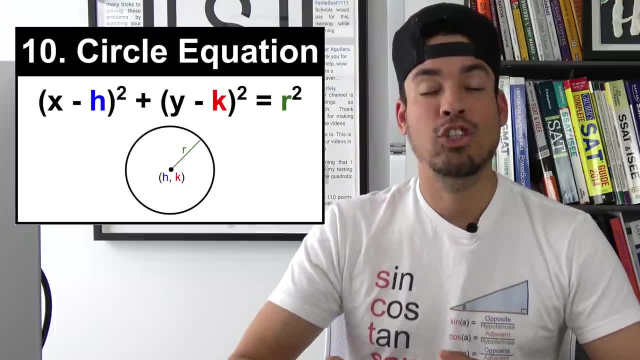 circle. They always seem to throw one or two test questions about circles and the equation and a coordinate plan on the test. So you want to know that R stands for the radius and H and K are the X and Y coordinates of the center of the. 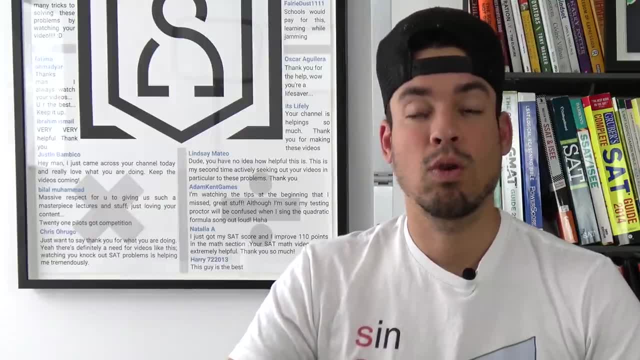 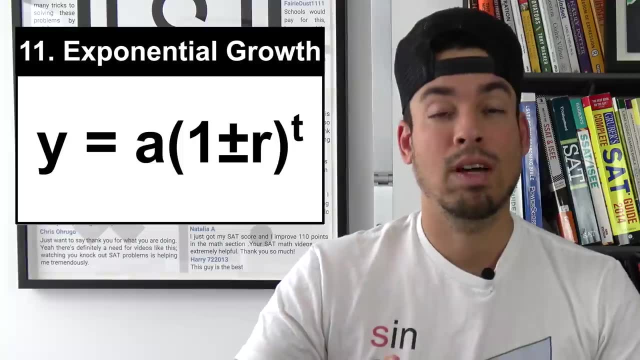 circle. Next on the list is the formula for exponential growth. Now, this equation is super important and will come into play if you get a question that says, hey, we've got a bank account, let's say, or we've got a population and we want to know how much money we're going to spend on the 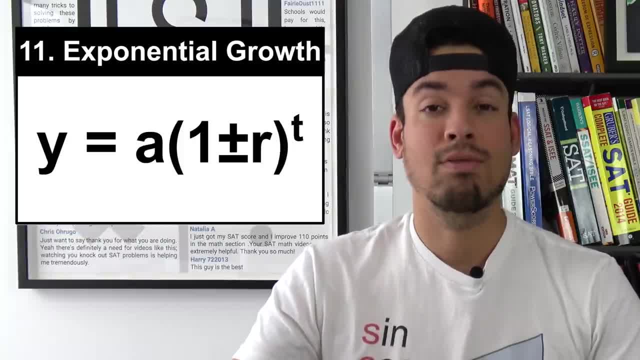 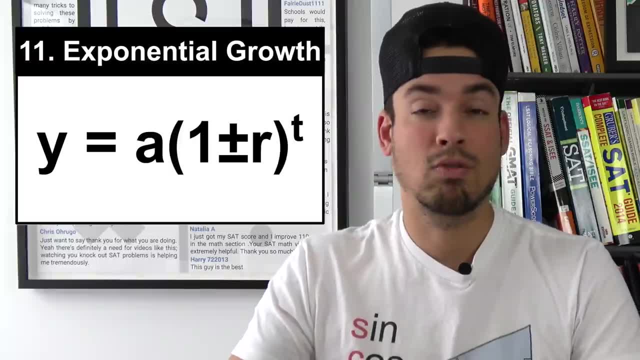 bank account. So let's say we have a population that's growing at 12% per year, every year. Where is it going to be in ten years? And so what these values are is R in that case would be the 12%. it's the amount it's growing Now. it could also be: 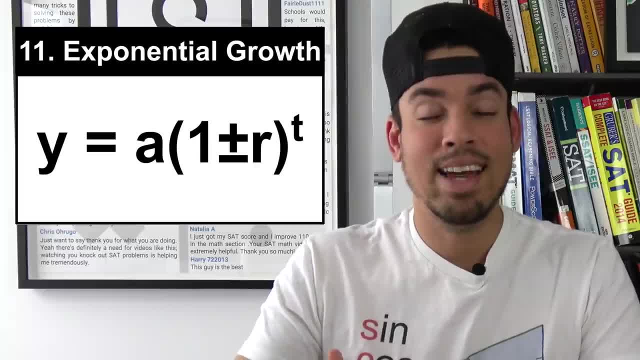 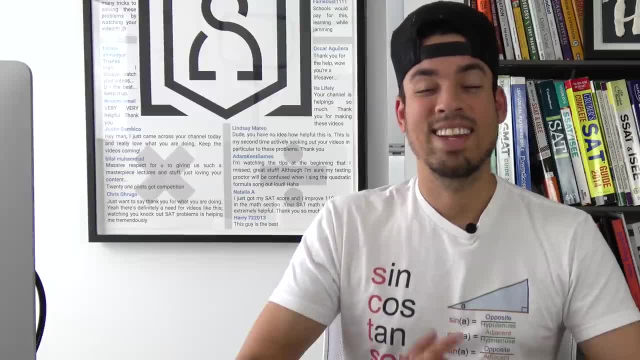 decreasing by 12%, It would still be 0.12, but then it's negative, so you are subtracting it in that case, And of course T stands for the number of years after the starting point. Next we have the formula for an arithmetic sequence. 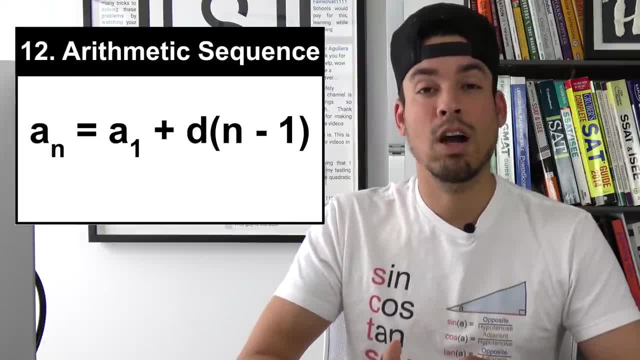 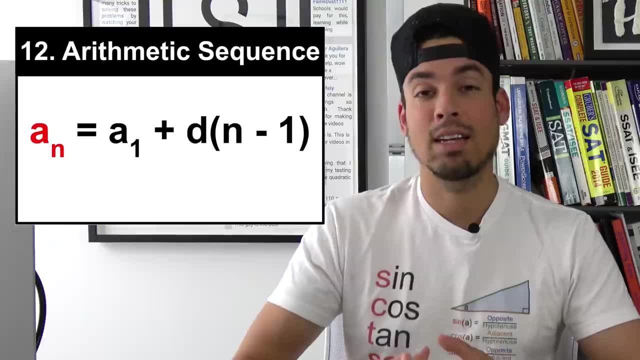 An arithmetic sequence is a sequence of numbers that either jumps up or goes, goes down, by the same amount each time, like two, four, six, eight, 10, et cetera. Now, in this sequence, a sub n is a of the nth term. 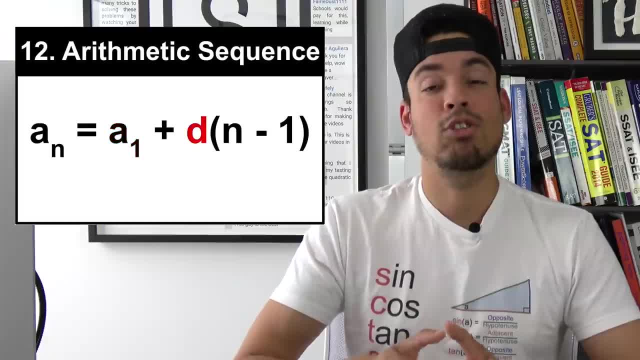 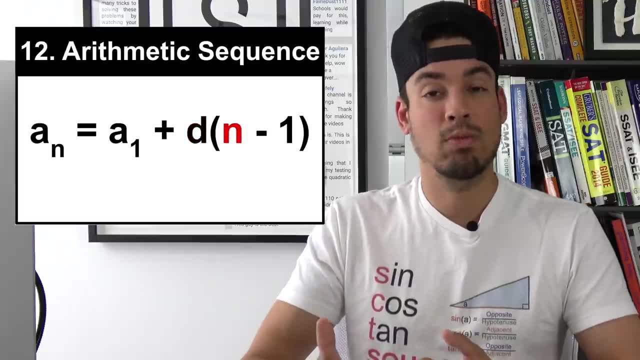 equals a sub one, which is the first term, plus d, which is the common difference. like the example I gave you, two would be the common difference times n minus one, and n is the term that you're trying to find. 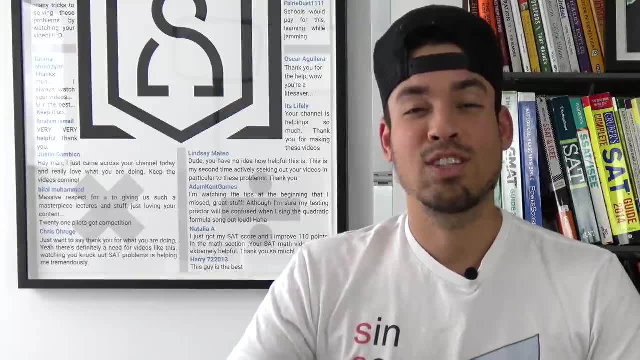 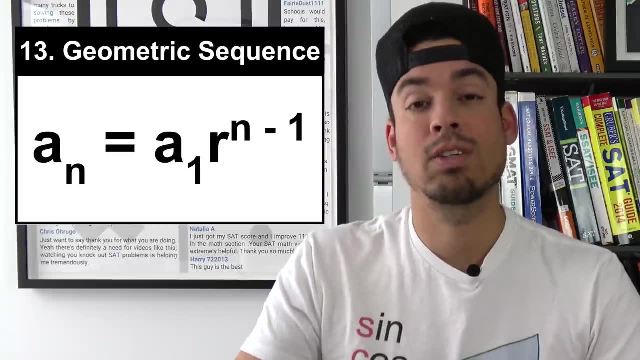 Like, if you're trying to find the 100th term, you'd plug in 100 for n. Next we've got the formula for a geometric sequence. Unlike an arithmetic sequence, a geometric sequence progresses by a multiplier. So, for example, if you have a multiplier of three, 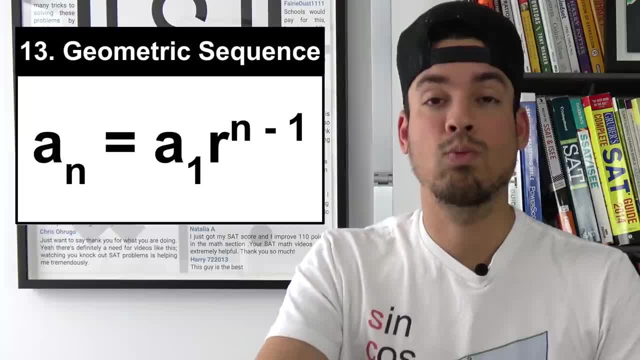 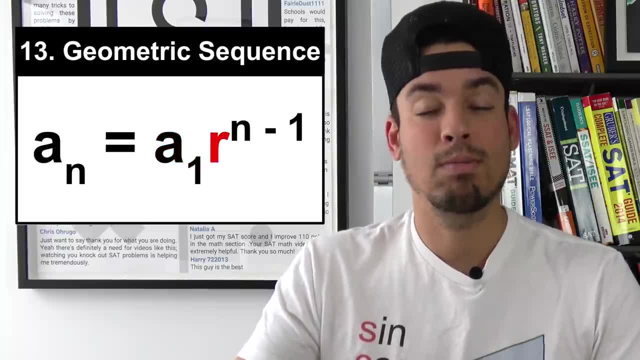 it would go three, nine, 27,, 81, and so on and so forth. So in this formula, again, a sub one is the first term in the sequence, r is that common multiplier or common ratio, and then of course n is the term or number of term. 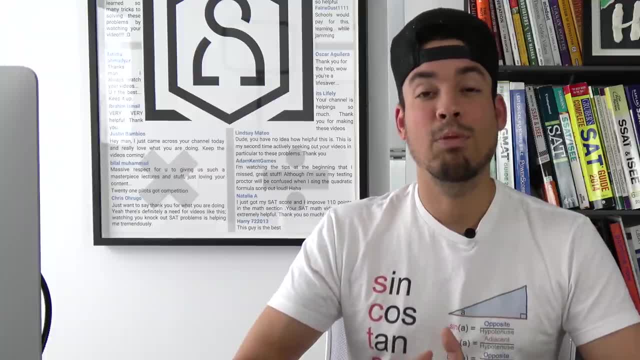 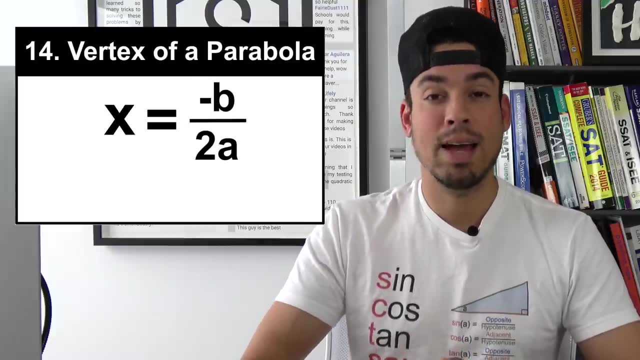 that you're trying to find. Next, we have a quick and easy formula to help you find the vertex of a parabola, and this is especially important if you're ever given a quadratic function and you're trying to find either the max or min value. 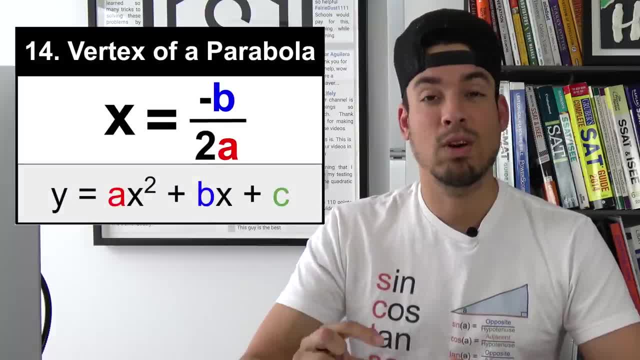 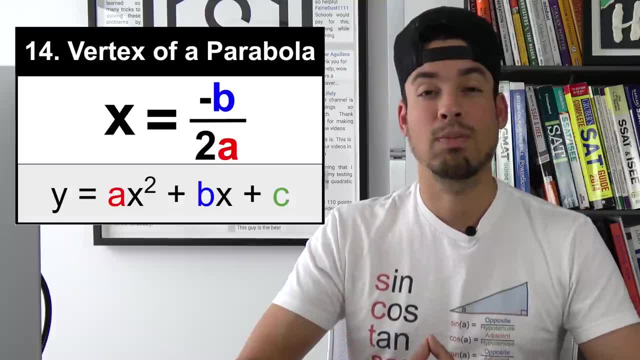 You can quickly plug this in and negative b. so b stands for, again, the coefficient of the second term in the quadratic and that a value is from the coefficient of the first term in the quadratic. Next on the list is how we convert. 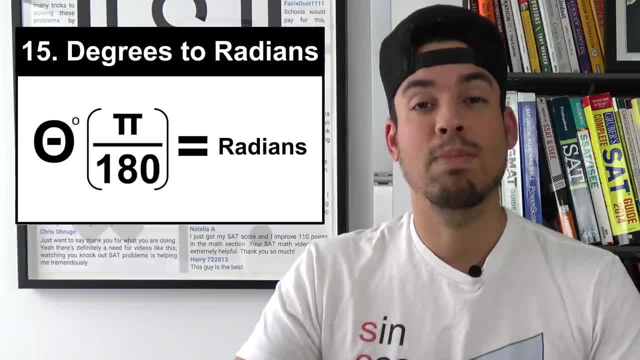 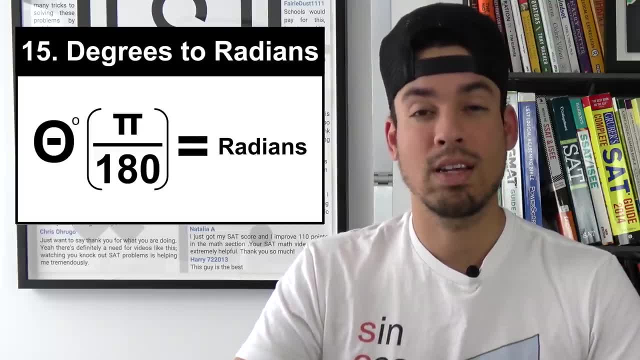 from degrees to radians. So all you gotta do is take your measurement in degrees, plug it in for theta, multiply it by pi over 180, and you get the equivalent value in radians. Next on the list is vertex form of a parabola. 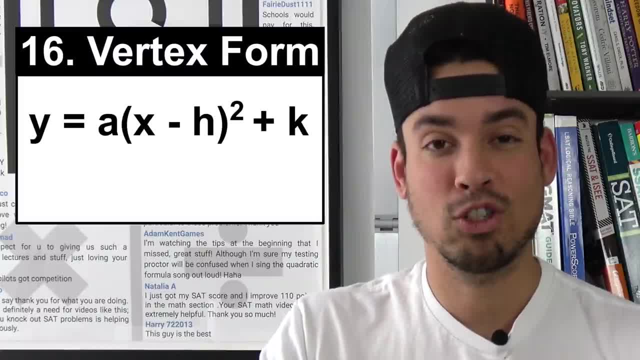 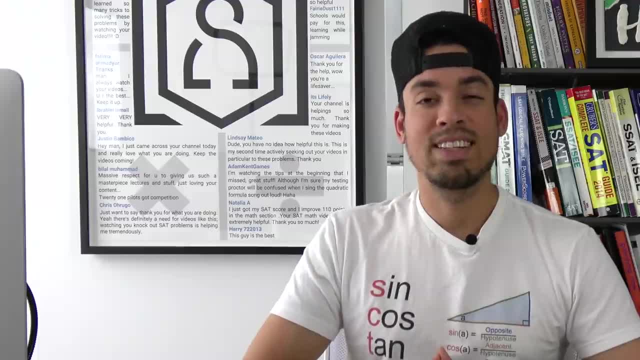 This is a great formula to have in your back pocket, because if you see a quadratic function presented in this format, you can quickly see where the vertex is. The vertex is at h comma k. Finally, one of the most famous formulas in math: Pythagorean's theorem. 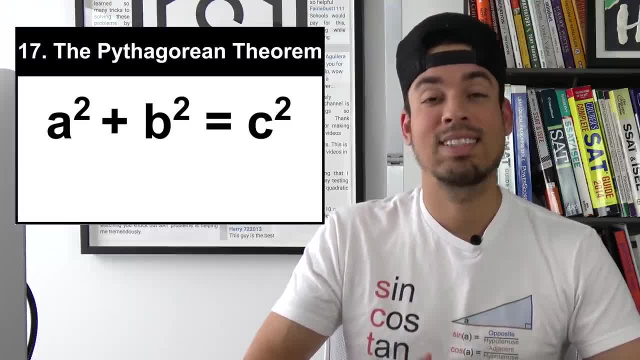 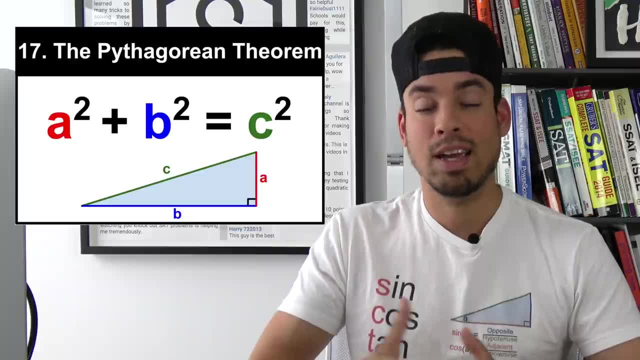 It's not that difficult of a formula to memorize. You should really have it down. It's: a squared plus b squared equals c squared. for any right triangle, where c is the measure of the hypotenuse, a and b could be either leg.